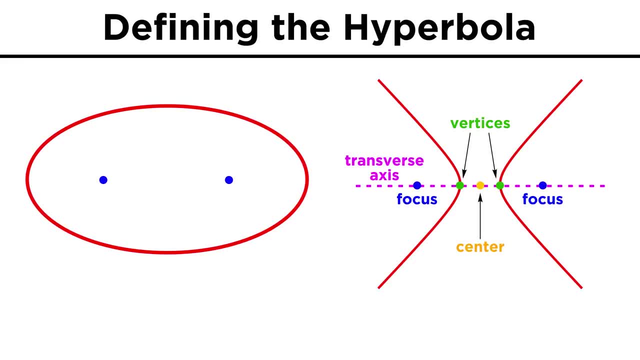 The center, which sits on the transverse axis that connects the vertices, The equation for a hyperbola will be extremely similar to that of an ellipse. In fact, the only difference is that instead of a plus here we have a minus, which makes 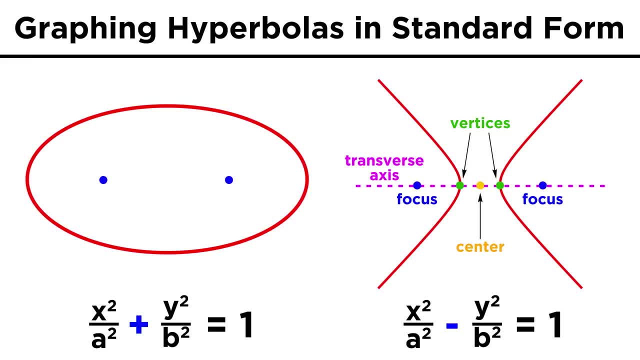 sense, given the difference between distances to the foci being constant instead of the sum, Everything else will be the same, except that for an ellipse we always put X to the center. So we always put X squared first and Y squared second, while the A and B terms could move. 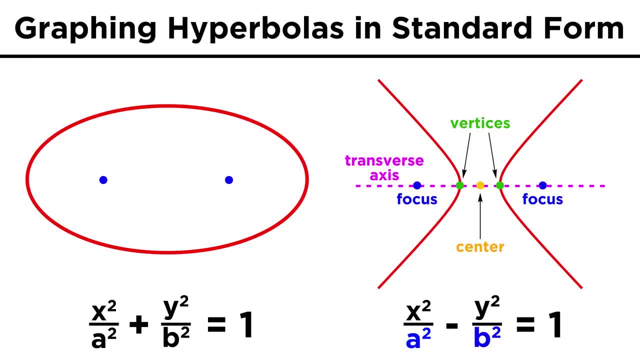 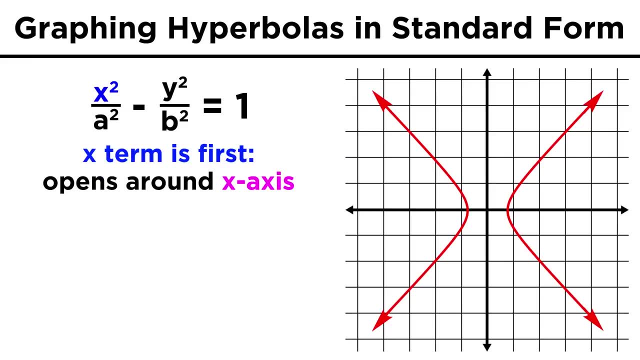 around This time, the A and B terms will stay put, while X and Y can swap spots. If it's the X term first, the hyperbola will open up around the X axis. If the Y comes first, it will open up around the Y axis. 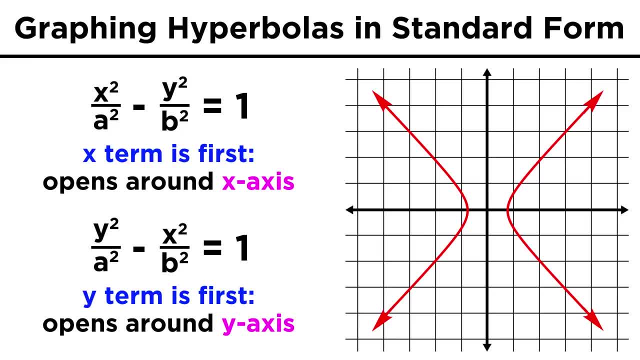 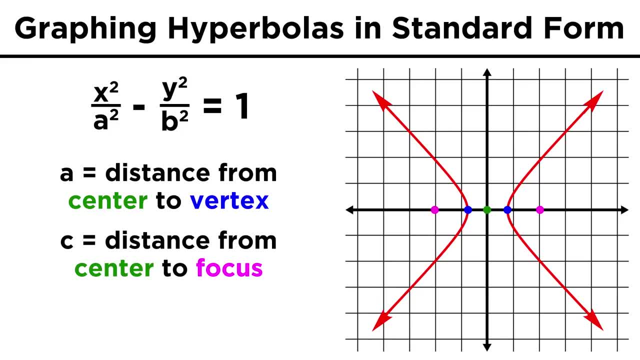 The A, B and C terms we know will mean pretty much the same things as well. Okay, So A is the distance from the center to a vertex and C is the distance from the center to a focus. One difference is that B no longer means much graphically and we will just use it to solve. 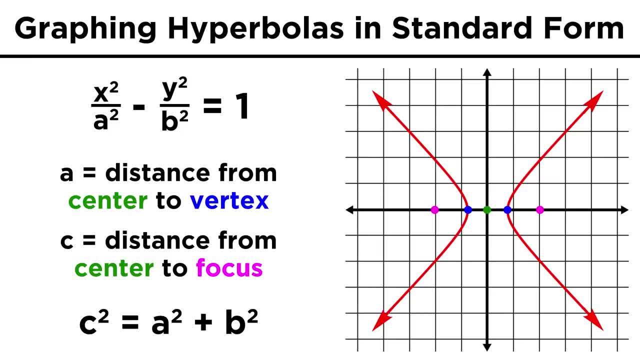 for A or C, and this time the equation will be: C squared equals A squared plus B squared. Let's try an example. Here's an equation in standard form where A squared is sixteen and B squared is nine. Let's try an example. 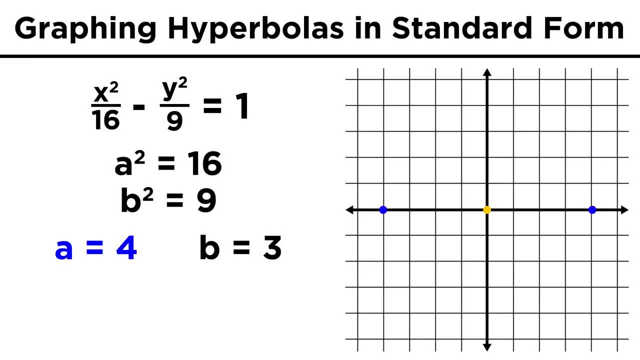 A is the distance to a vertex, so the vertices must be at plus and minus four. Then we do C squared equals sixteen plus nine or twenty-five, so C is five and the foci must be at plus and minus five. And that's enough information to do a rough sketch of the hyperbola. 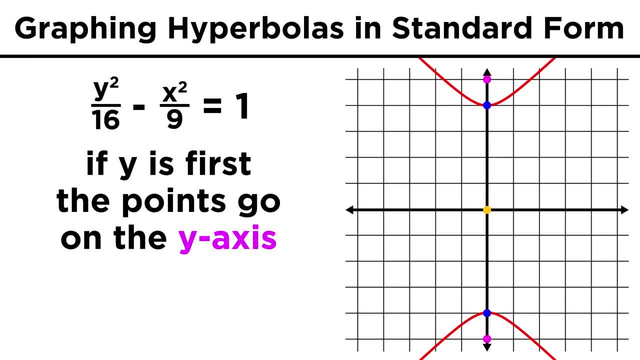 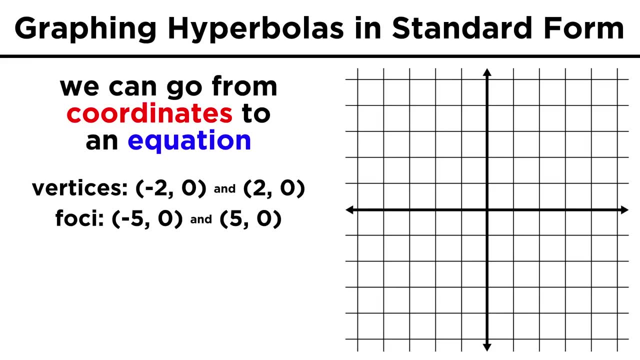 If the X and Y terms were reversed, we would have a similar situation, except that now the transverse axis is reversed, A is vertical, but the distance to the vertices and foci will remain the same. Just like with ellipses, we can also be given coordinates for vertices and foci and generate 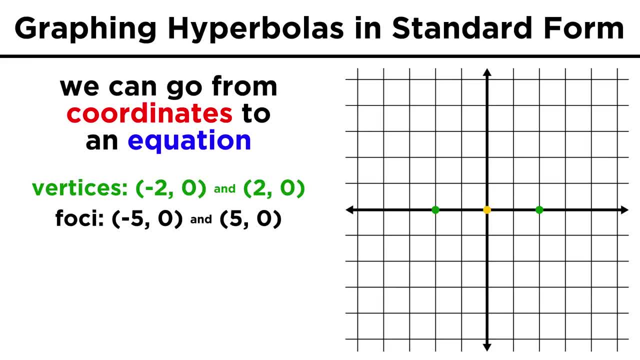 the equation from that Vertices on the X axis at plus and minus two, and foci at plus and minus five, means that twenty-five equals four plus B squared, which makes B squared twenty-one. Okay, Okay, So our A squared and B squared terms go here. 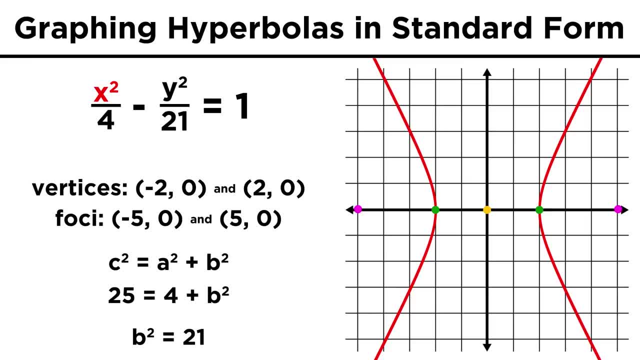 The X term comes first, since it's horizontal, and that's the equation for the hyperbola. If you're having trouble drawing the branches of the hyperbola, one thing that can help is to draw the asymptotes. These are the lines that the branches approach, getting closer and closer but never touching. 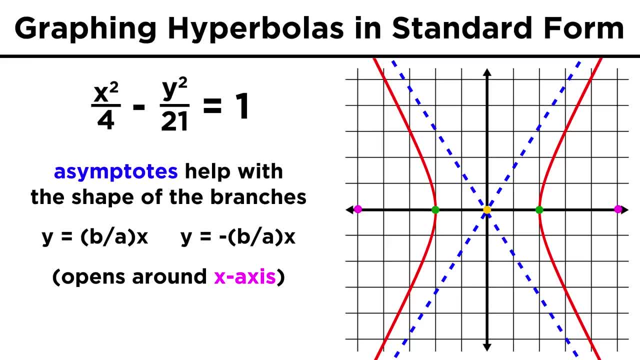 and for a hyperbola that opens around the X axis, these asymptotes are the ones that are given by the equations: Y equals B over A times X and Y equals negative B over A times X. For a hyperbola that opens around the Y axis, the asymptotes are given by the equations: 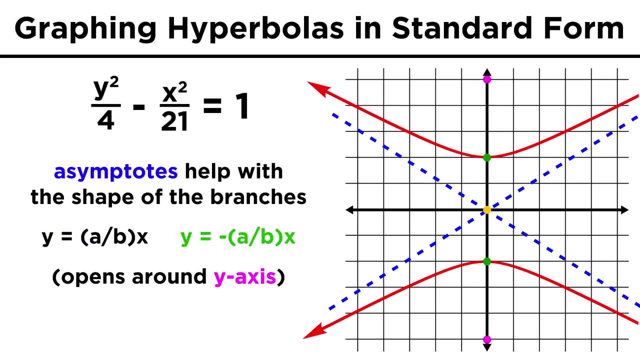 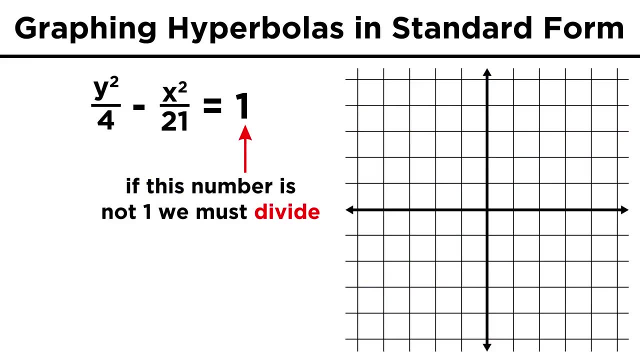 Y equals A over B times X and Y equals negative A over B times X. If you draw these asymptotes with dotted lines, they can help you draw the hyperbola a bit more accurately. Again, if a hyperbola is not in standard form, because this number is not one, we just divide- 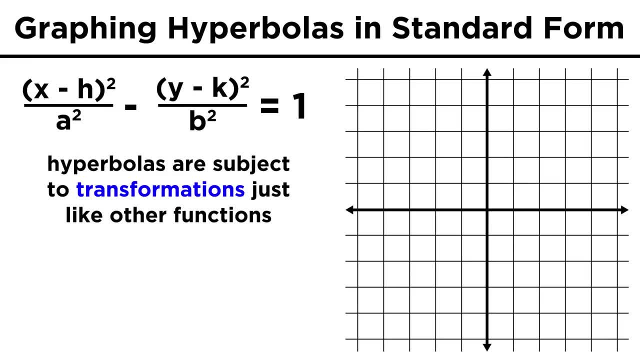 through by that number to get rid of it. And finally, hyperbolas can be transformed similarly to ellipses. If we rewrite as X minus H and Y minus K, the point HK will be the new center of the hyperbola. 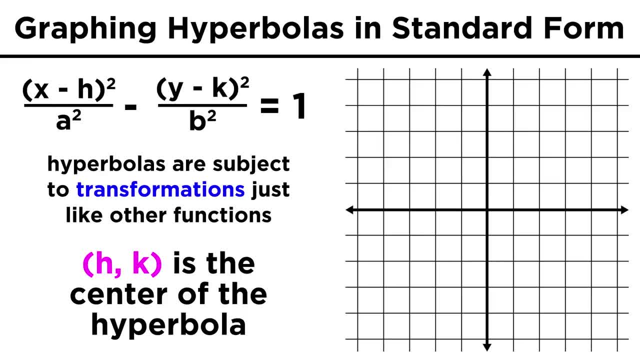 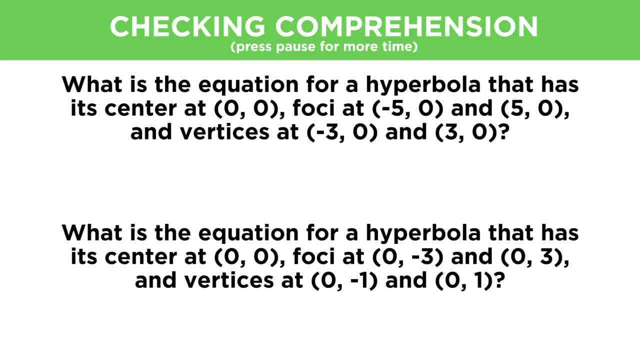 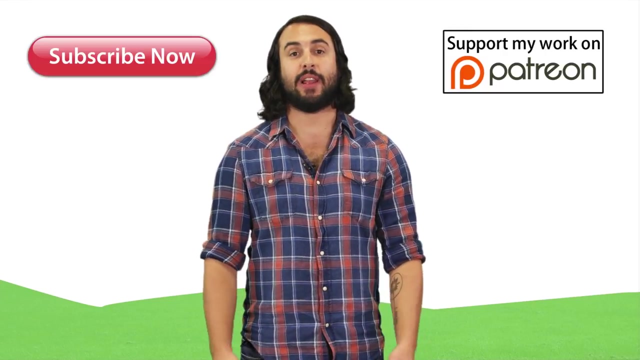 That's what we need to know about hyperbolas, so let's check comprehension. Thanks for watching. Subscribe to my channel for more tutorials, support me on patreon so I can keep making content and, as always, feel free to email me professordaveexplains at gmail dot com.